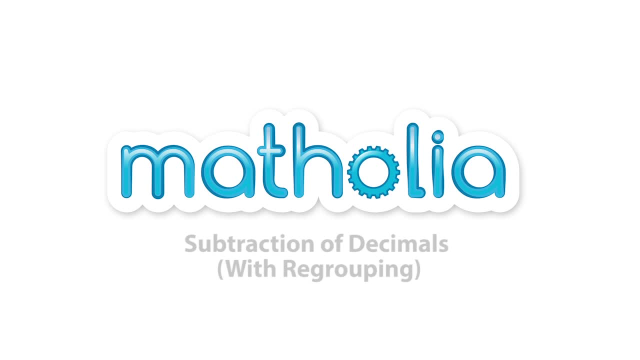 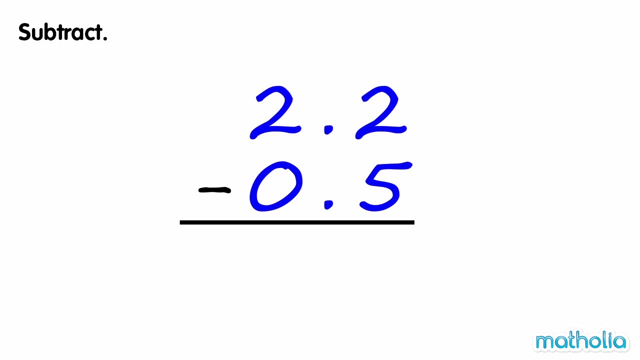 Subtract: Find 2.2 minus 0.5.. Start by subtracting the tenths. We cannot subtract 5 tenths from 2 tenths, So we regroup 1: 1 into 10 tenths. We now have 12 tenths. 12 tenths minus 5 tenths. 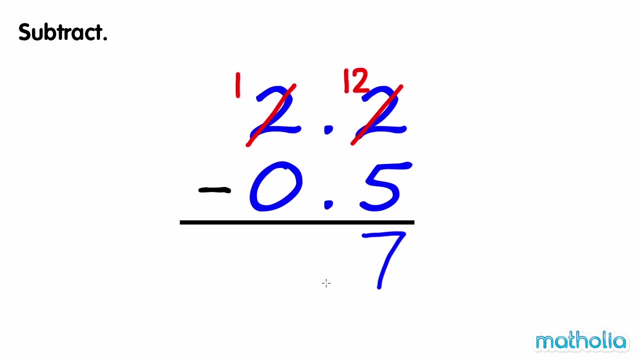 equals 7 tenths. Write the decimal point Now subtract the ones 1: 1 minus 0 ones equals 1, 1.. So 2.2 minus 0.5 equals 1.7.. Subtract, Find 3.47 minus 1.59.. Start by subtracting the hundredths. We cannot subtract. 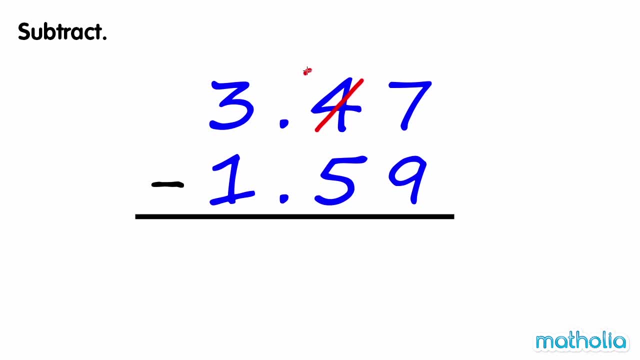 9 hundredths from 7 hundredths. So we regroup 1 tenth into 10 hundredths. We now have 17 hundredths. 17 hundredths minus 9 hundredths equals 8 hundredths. Subtract the tenths. 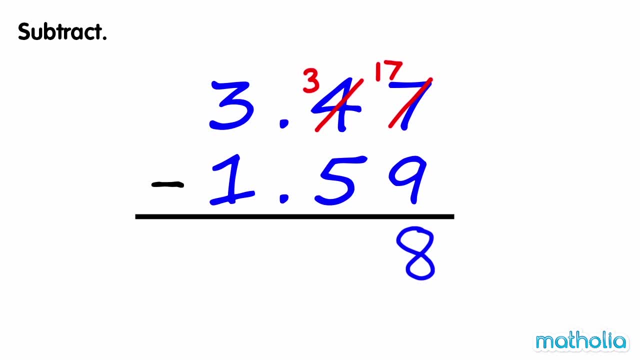 We cannot subtract 5 tenths from 3 tenths, So we regroup 1 tenths from 3 tenths. So we regroup 1, 1 into 10 tenths. We now have 13 tenths. 13 tenths minus 5 tenths equals 8. 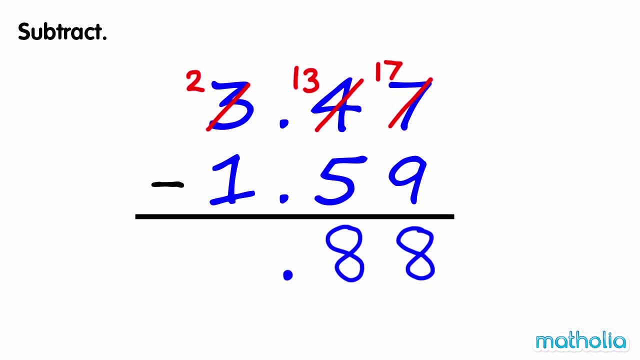 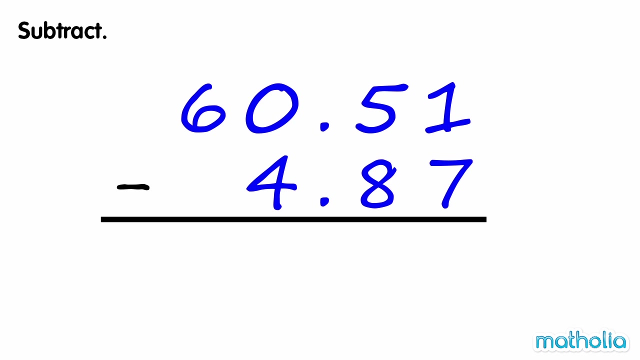 tenths. Write the decimal point. Subtract the ones, 2 ones minus 1, 1 equals 1, 1.. So 3.47 minus 1.59 equals 1.88.. Subtract, Subtract Subtract Find 60.51 minus 4.87.. We cannot subtract 7 hundredths from 1 hundredth, So we regroup. 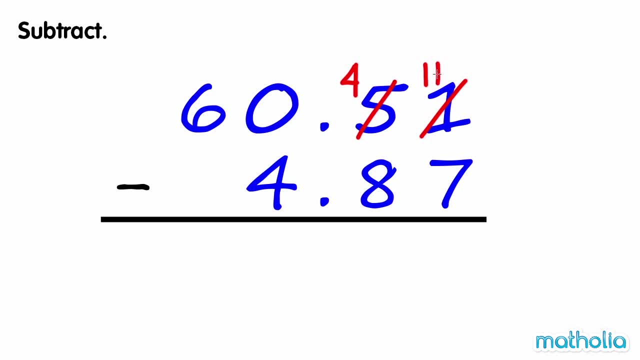 1 tenths into 10 hundredths, We now have 11 hundredths. 11 hundredths minus 7 hundredths equals 4 hundredths. Subtract the tenths. We cannot subtract 8 tenths from 4 tenths.